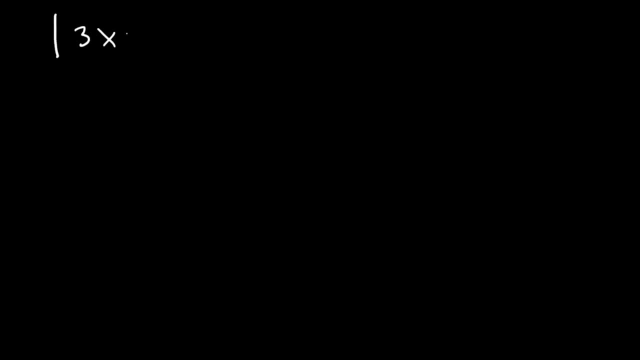 Now, what if we have an absolute value expression with an inequality? What do we need to do? Well, we still need to write two equations. The first one is going to remain the same. Now for the second one, we need to do two things. We need to change the positive 5 to a negative 5,. 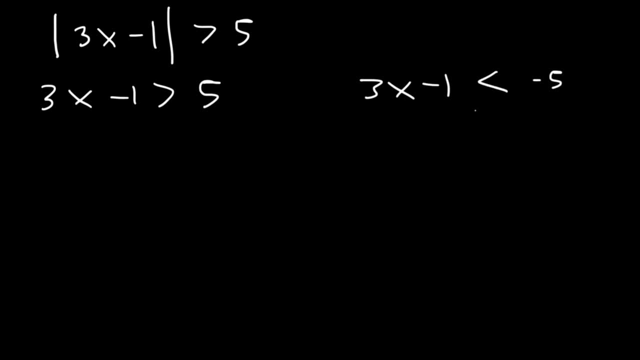 and we need to change the direction of the inequality. So that's important. Make sure you understand that, And then after that just solve it: 5 plus 1 is 6, and then let's divide by 3.. So x is greater than 2.. Now for the other one, negative. 5 plus 1 is negative 4.. And if we 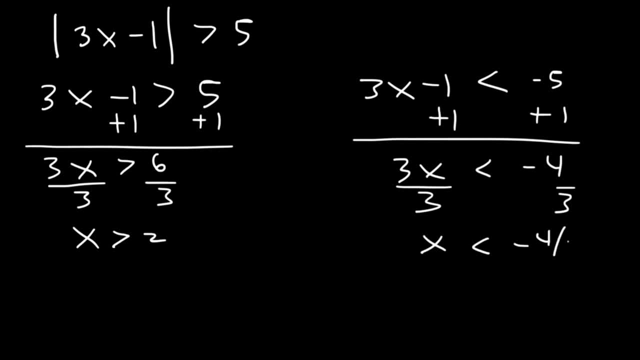 divide it by 3, we're going to get a fraction. x is less than negative 4 thirds. Now, because we're dealing with inequalities, we need to plot the solution on a number line, So we need 2.. Negative 4 thirds is about negative 1.3,, which is between negative 1 and 2.. 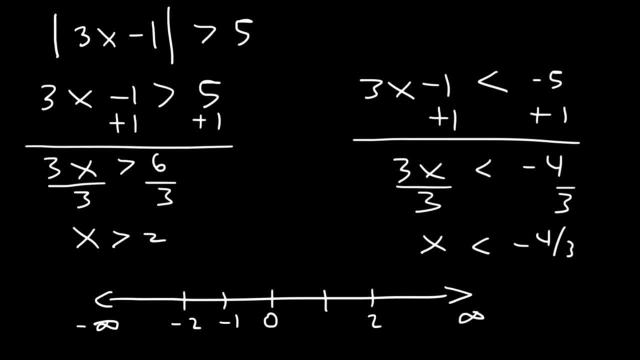 So x is greater than 2, which means that we have an open circle at 2, shaded towards the right, And x is less than negative 4 thirds, which is about negative 1.3.. So it's an open circle. 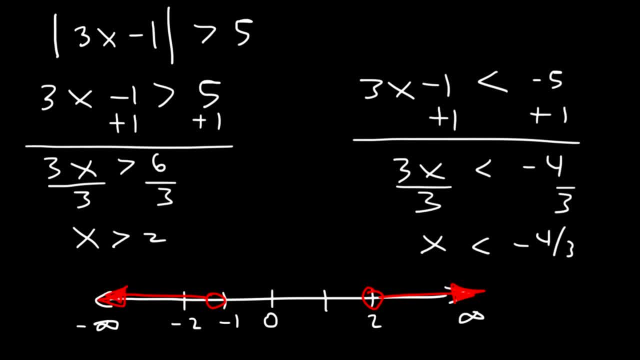 shaded towards the left. Now the solution using interval notation. let's write it up. It's going to be negative infinity to negative 4 over 3, and then union 2 to infinity. So here's the 2 to infinity part and here's the negative infinity to negative 4 thirds. The open circle is: 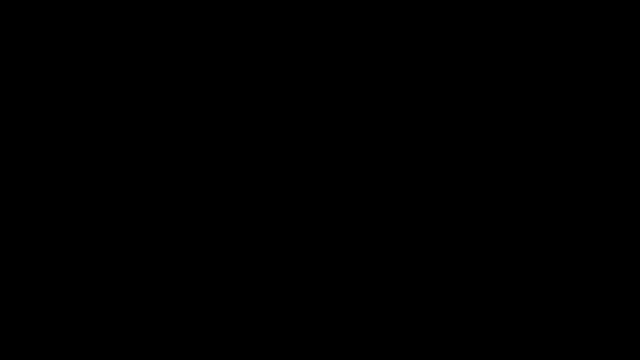 at negative 4 thirds. Just keep that in mind. Let's try another example. Feel free to pause the video and work on it Now. right now we can't write two equations yet. We need to get the absolute value expression on one side of the equation first. So first let's subtract both sides by 3.. So what we're?